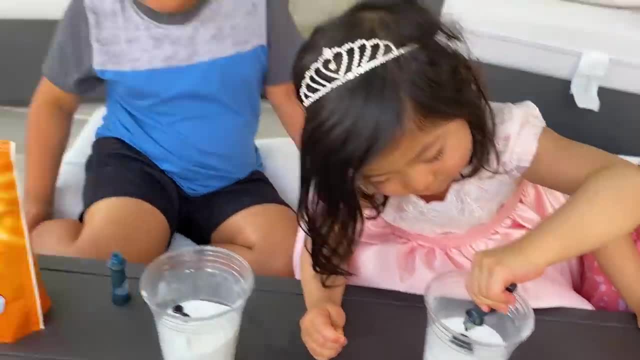 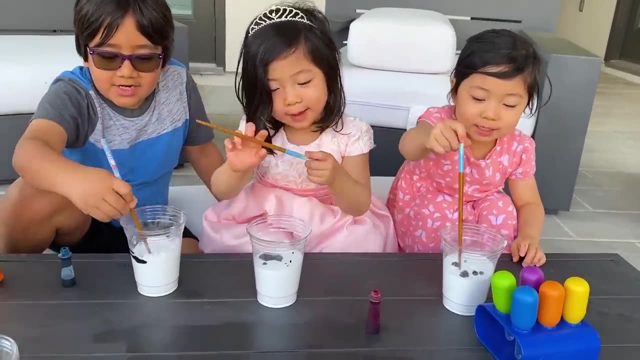 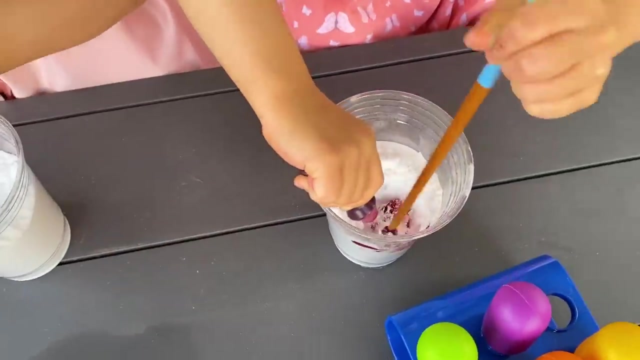 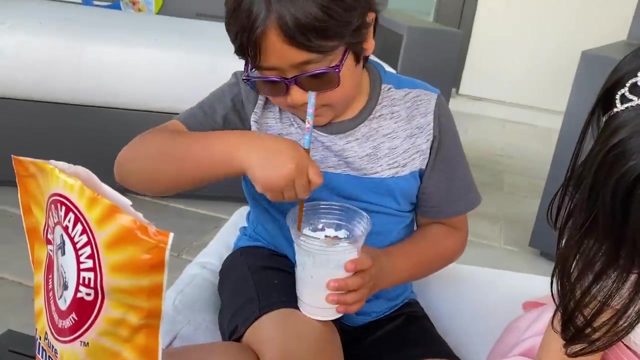 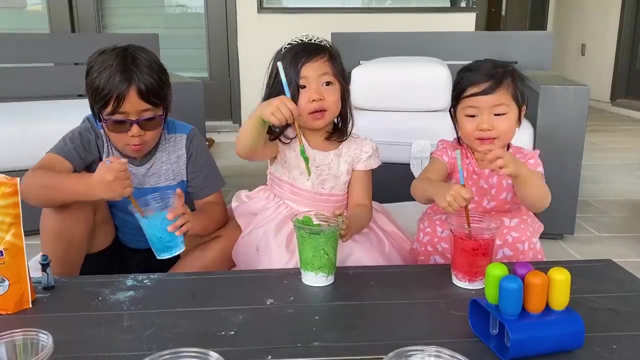 Kate did some red, Emma did some green and Ryan did blue. Next, you're going to need to agitate to get something to agitate. Good girls, Good Emma, Good Ryan. Look guys, mine's almost fully blue. Wow, yeah, Keep agitating. Good, I'm going to mix in a little more. I'm going to mix in a little more. 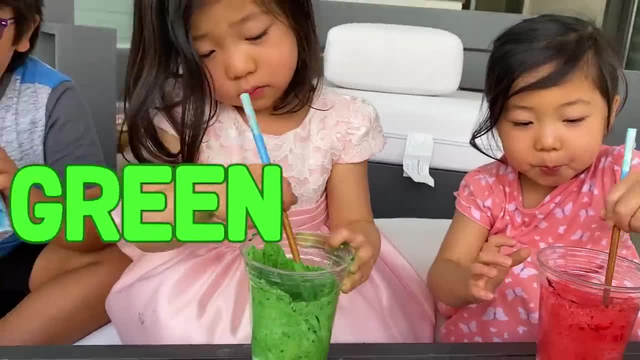 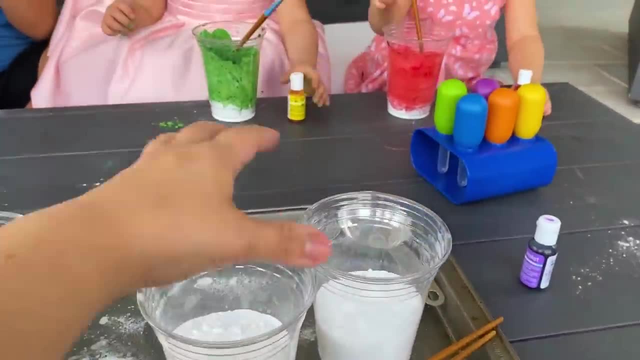 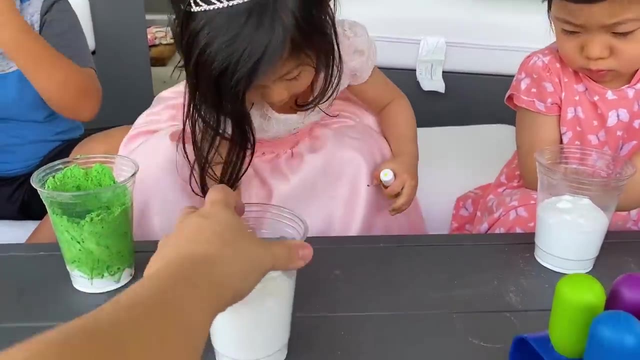 Yeah, so you guys, colors are coming good See: Red, green, Green and blue. Good girls and boys. Okay, so we're done with our three cups. Now we're going to do these three. Okay so Kate's going to do orange and then Emma's going to do yellow and then Ryan's. 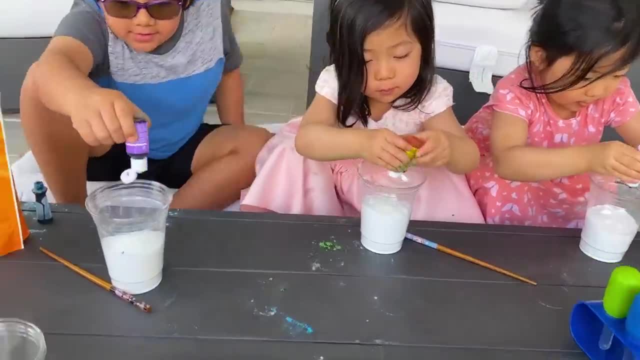 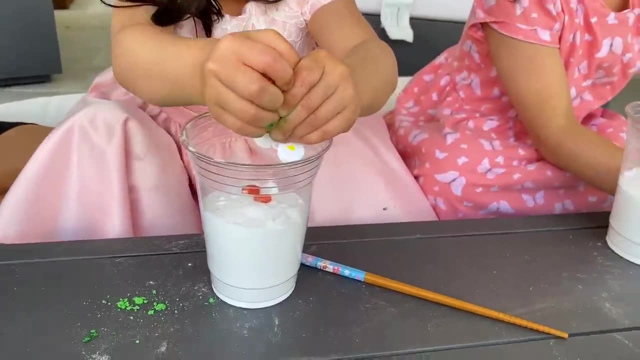 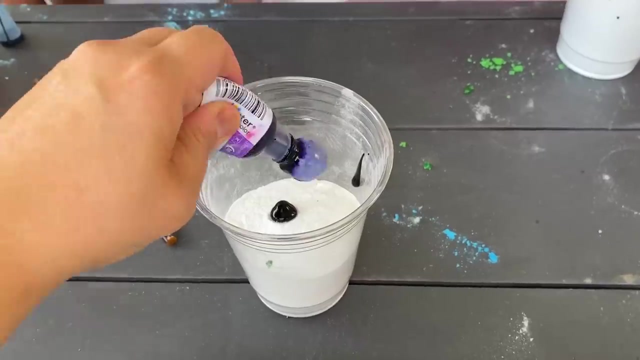 going to do purple. Good, There you go. Add your color Purple. It still doesn't look like yellow. It will. Good, There you go. Yellow. Kate got her orange. Okay, there, it is Purple's out, but it's okay. Look at the bubble. Look at that giant purple bubble. 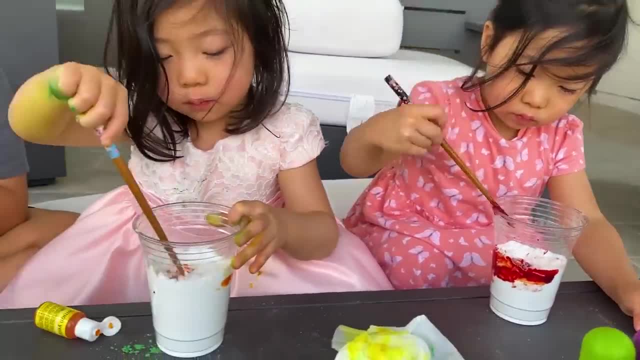 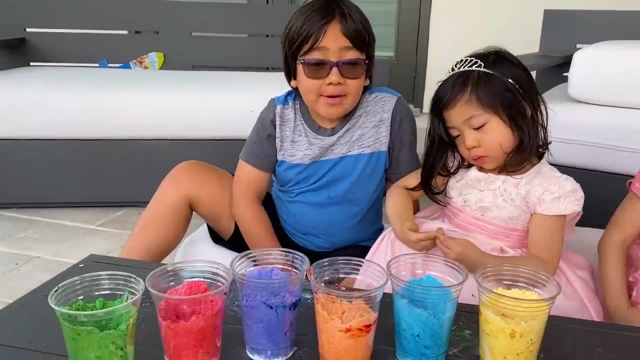 All right, start agitating. There you go, Agitate, agitate, Agitate, agitate, agitate, agitate, agitate. Okay, we got our rainbow colors. Nice Okay, guys. so now we're going to pour all the colors. 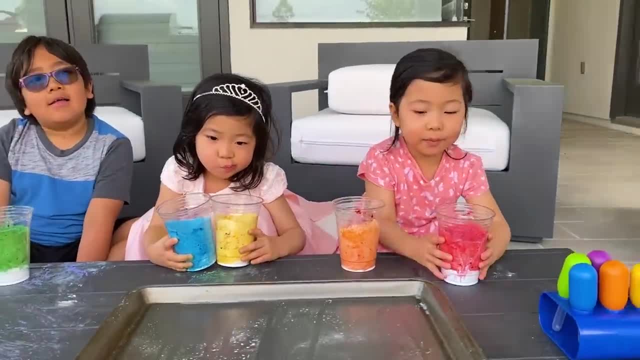 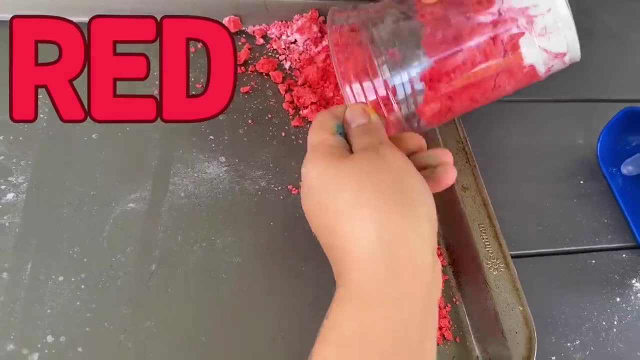 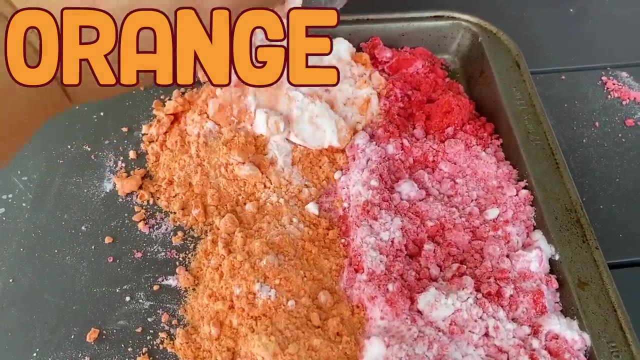 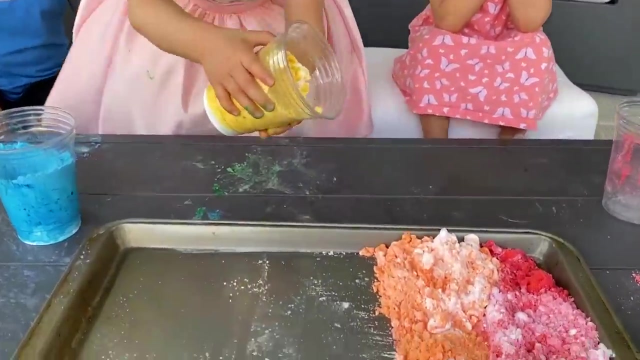 into this pan here. So, Kate, you can start first with red, Pour it in. Yeah, There we go. Okay, we got our red and now we're going to do our orange. All right, there we go. Orange. Ooh, nice, Good job, Kate, Let's go. There you go. Good, I help you, It's okay. There you go. 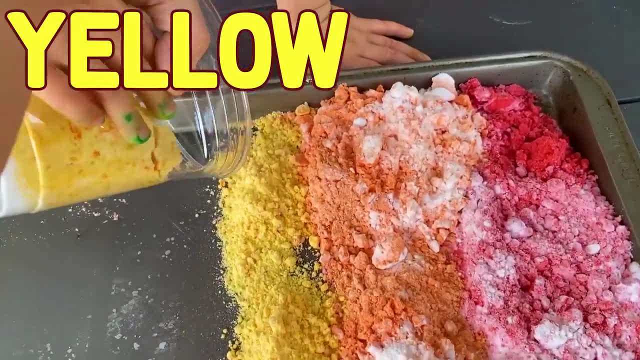 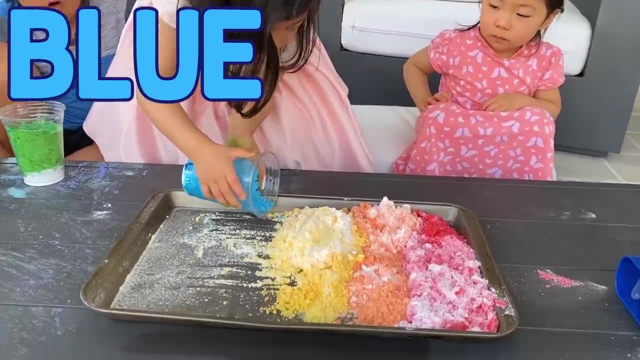 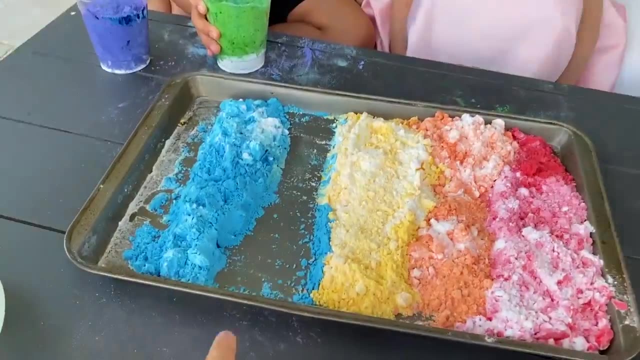 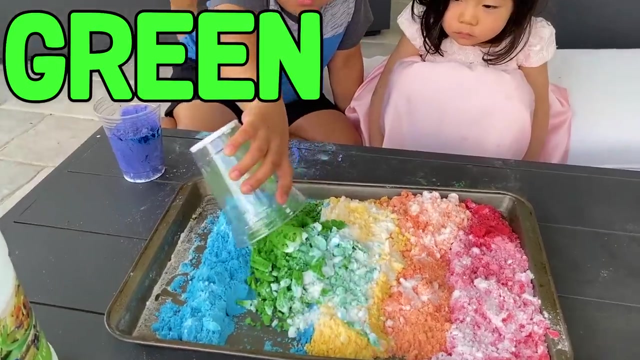 Good girls. Wow, So beautiful. huh, Yeah, it's like a rainbow. Yeah, Now we do blue. Good, There you go. Yeah, beautiful, Okay, so we accidentally forgot the green here, so Ryan's going to pour the green. Yeah, There we go. Whoa, It's okay, We can fix it, Spread out. 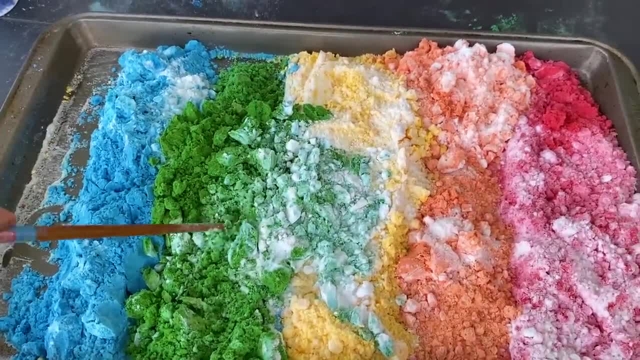 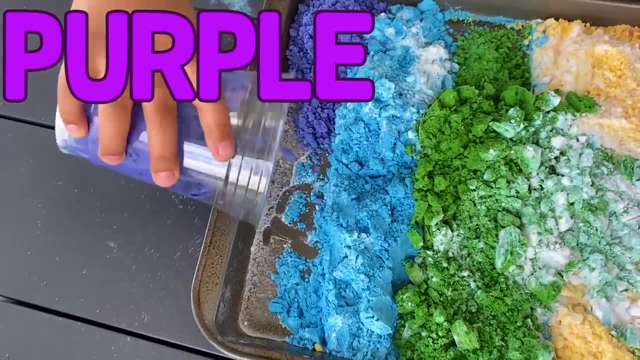 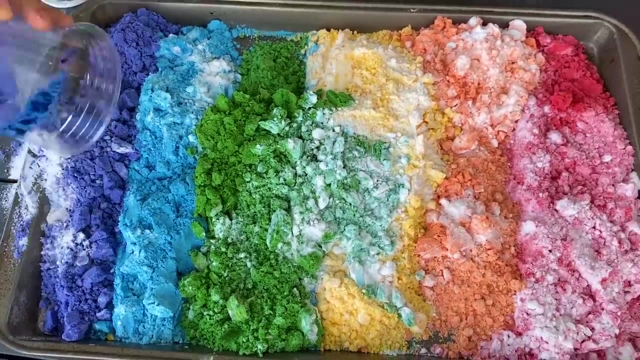 the green. It looks pretty. huh, Yeah, It's actually a lot of green. Yeah, It's like a rainbow, but now we need purple. That's right, purple. Yeah, Wow, So beautiful. It looks like a rainbow. It does. Now mom can do these. Yeah, Almost done. 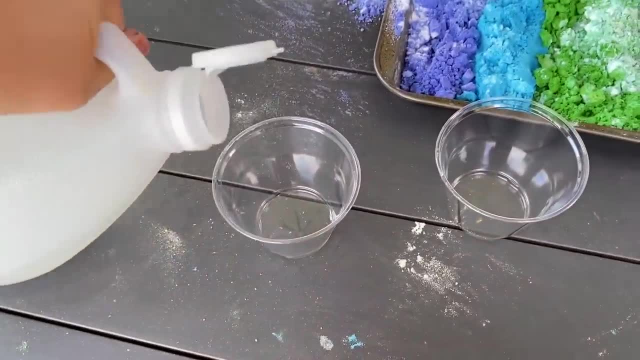 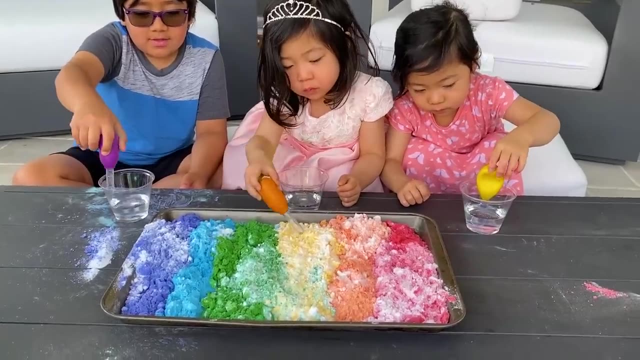 Good job, guys. You're going to need some vinegar here. Can you help me? Yeah, of course. Okay, I'm going to pour some vinegar in each cup for you guys. Okay, there you go, Pick up some vinegar and then just do it. Yeah, I'm going to squeeze Like this. You see the bubbles, Emma, look. 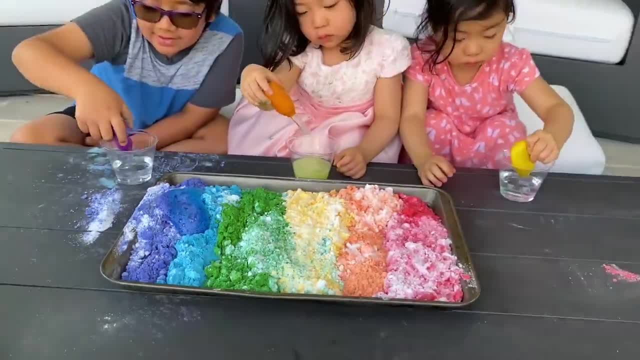 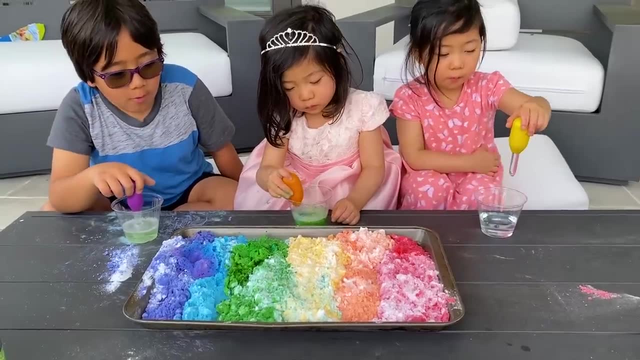 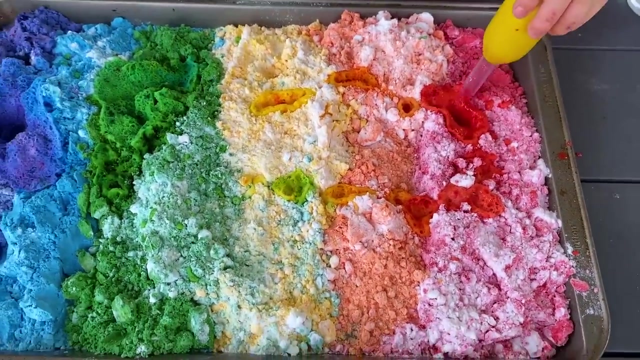 Whoa, Kate, look, I put some bubbles. Are we going to mix it into the cup? Whoa, Whoa, Whoa, Look, mine is even getting taller. Wow, And it's already cold. Same time, Yeah, Mine is growing. 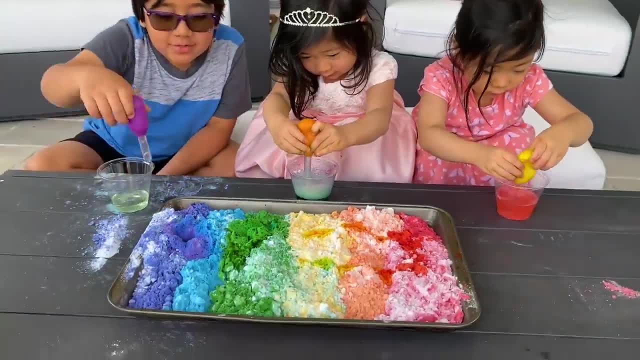 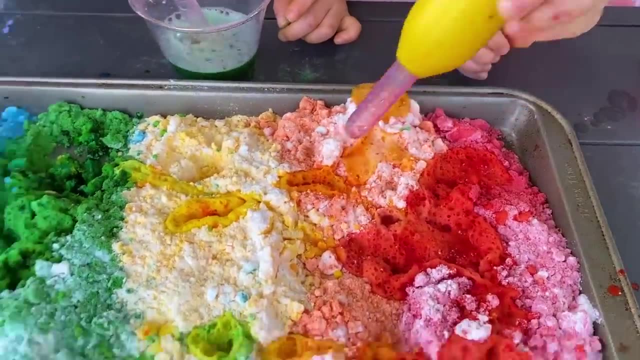 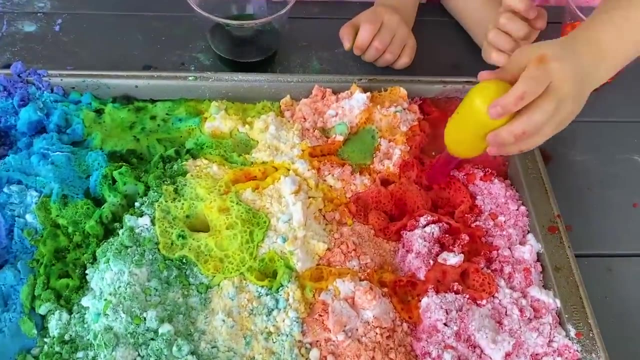 And that's just mixing over there. Wow, Okay, Mine's just mixing together. Whoa, Whoa, Whoa, That's a big one. I have a reaction inside my cup. Whoa, Whoa, That's cool. 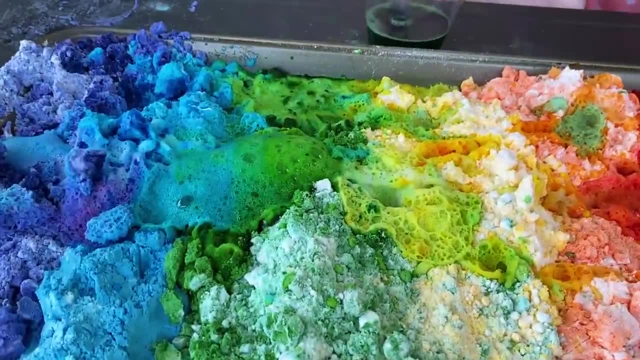 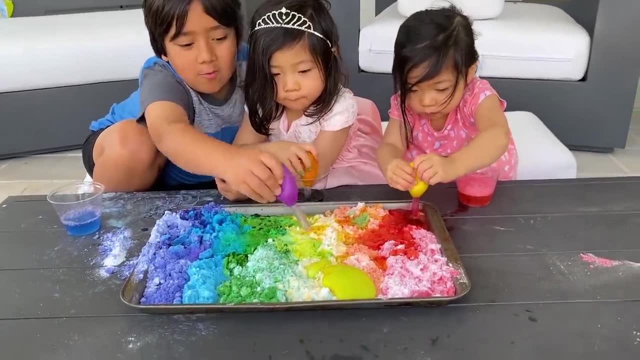 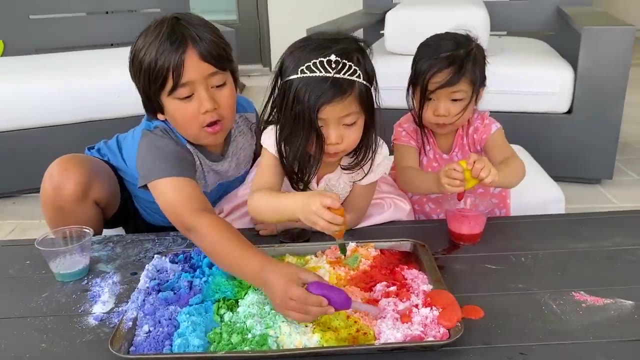 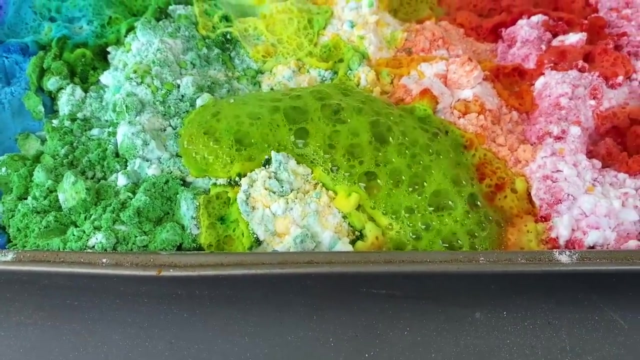 Whoa, There's a spot you guys haven't done yet. Okay, I'm gonna do it on one single spot. Okay, Whoa, that's giant. Another one, Whoa, Is this the one with what? Yeah, Whoa, look at the bubbles. 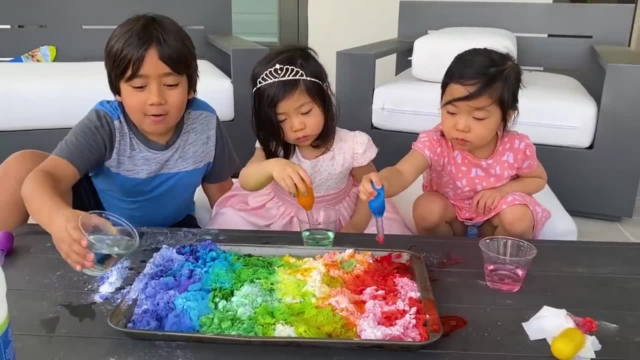 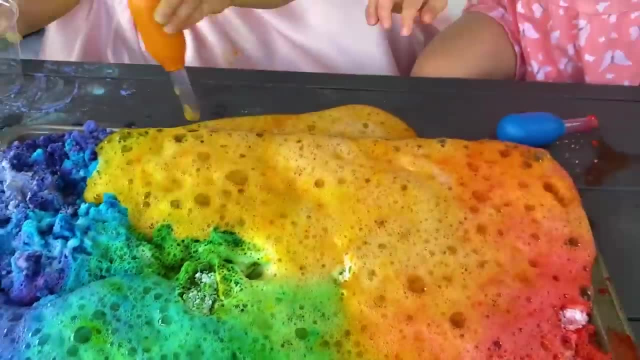 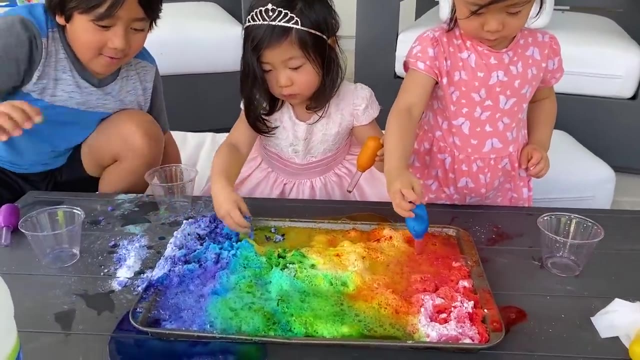 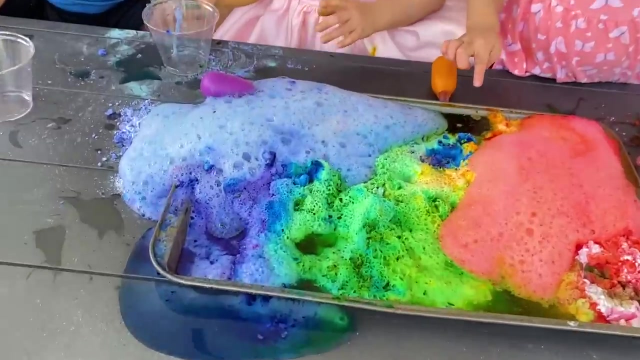 Okay, Okay, we're gonna pour it now. Whoa, Whoa, Rainbow, Can I touch it? Yeah, Whoa, It looks so cool. That was fun. huh, Whoa, Whoa, Can I touch it?